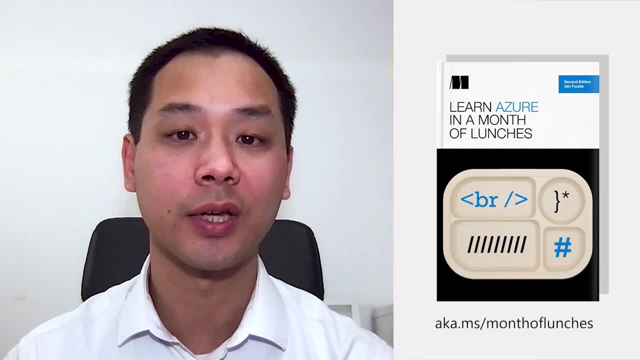 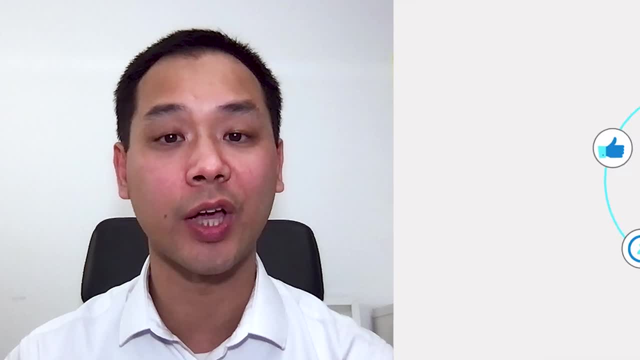 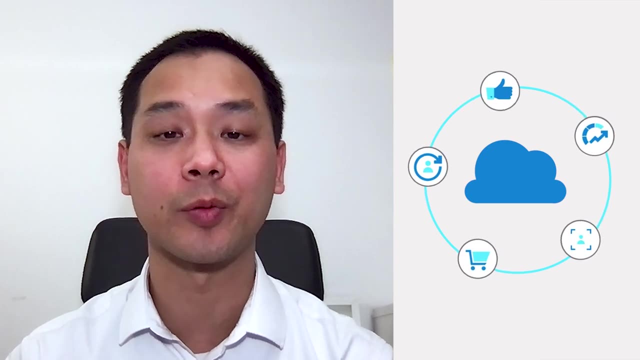 You can download this ebook for free at akams slash monthoflunches. For today's demonstration, I want to show you Azure App Service, which is a web hosting service in Azure. that's great for web developers because it supports all the most popular programming languages that web developers use. 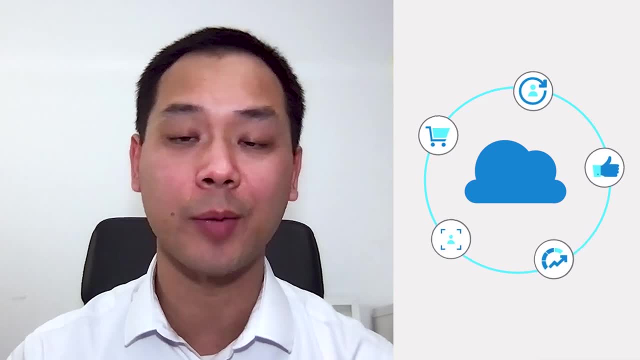 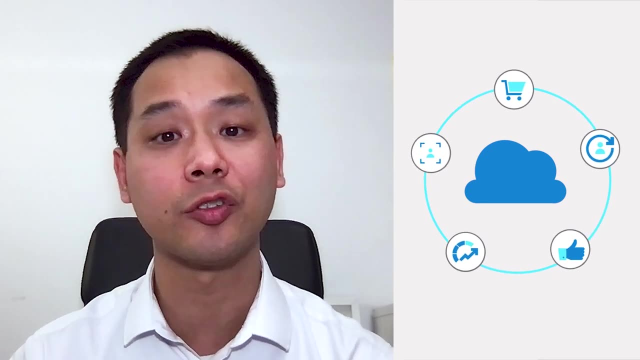 So we're going to create a resource group, we're going to create an app service plan and then we're going to create an app service app. After that, we're going to deploy a simple HTML page to Azure and then we're going to see it running live in Azure in minutes With that. 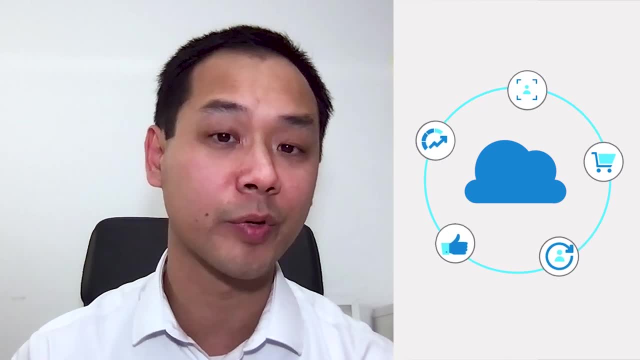 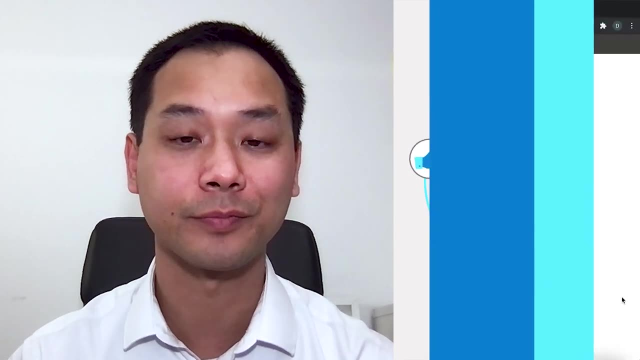 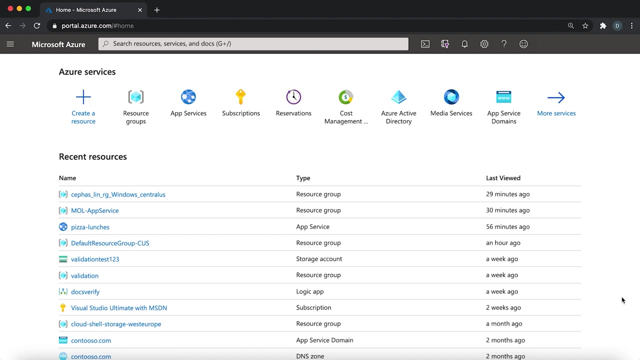 you get the benefit of security, high availability and scalability that Azure has to offer. So let's get to it. So to get started, open a web browser and navigate to portalazurecom And log in with your Azure account. And once you're logged in, you're going to see: 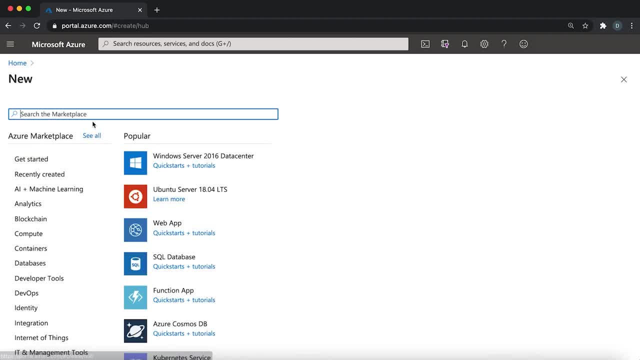 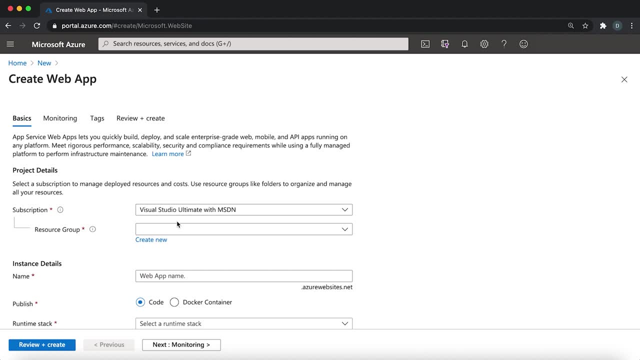 a home page like this And then go ahead and go to create a resource And then click web app. A web app is just an app service app And in this create page you can specify the resource group you want and the app service plan you want and then the app you want. But for 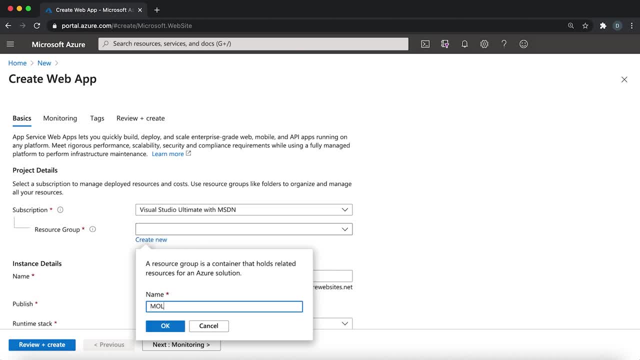 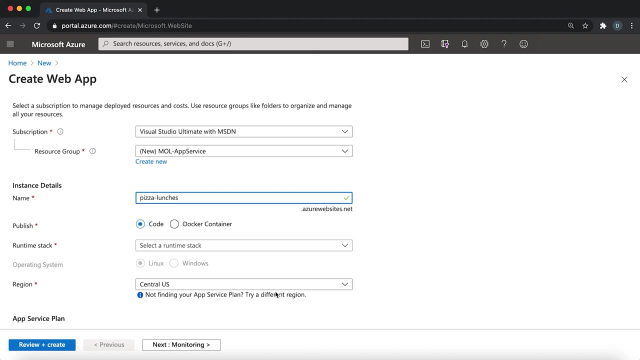 this video we're going to create everything, So let's create a resource group. Call it MOL for month of lunches app service, And then for the app name, let's give it a unique name called pizza lunches. Okay, And because you're just deploying HTML code, so let's stick with code. 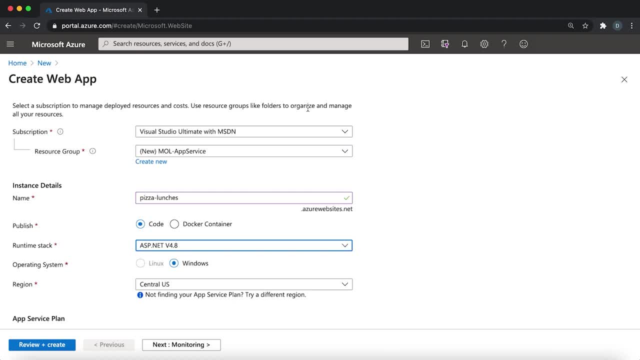 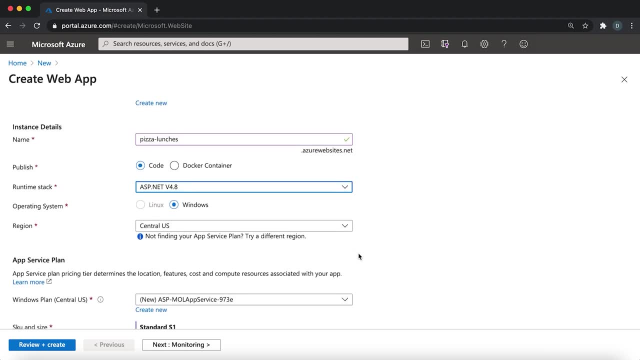 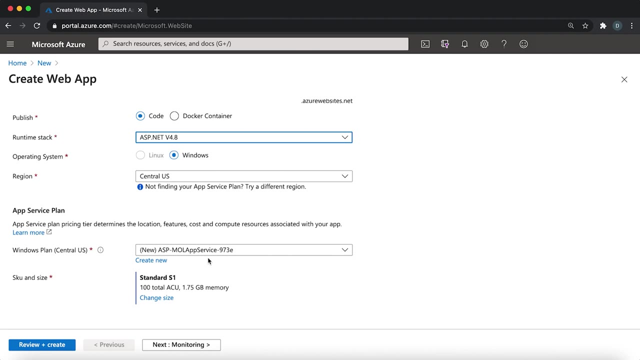 And for runtime stack, let's pick ASPNET 4.8.. You won't actually be running ASPNET 4.8, but that allows you to run your HTML code. Okay, Down to app service plan. you can see that a name is already generated for you. 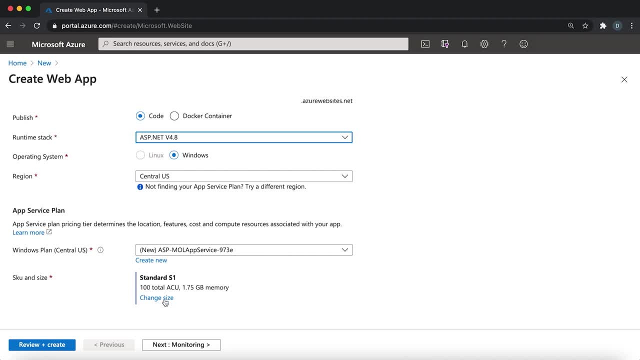 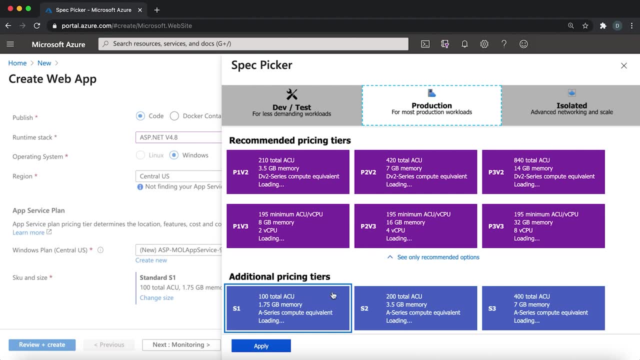 for a new app service plan And then for SKU and size, let's click change size And then for levitating. this is a high level option And you can see that this is the same HTML file, the name of the whole app. 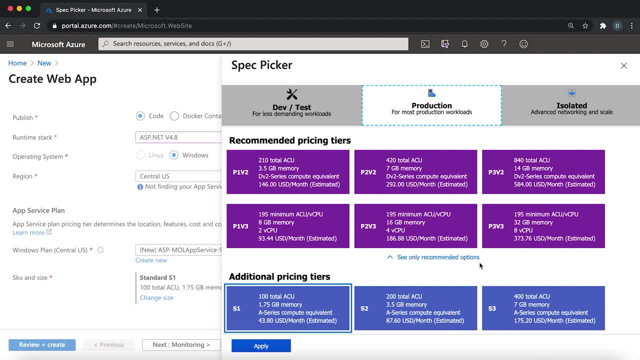 So again. so for the slide, the same code. So if you want to use the same button, you can use a different button from the previous slide. Okay, So let's go ahead and click save. So I'm going to change the name of this service plan. 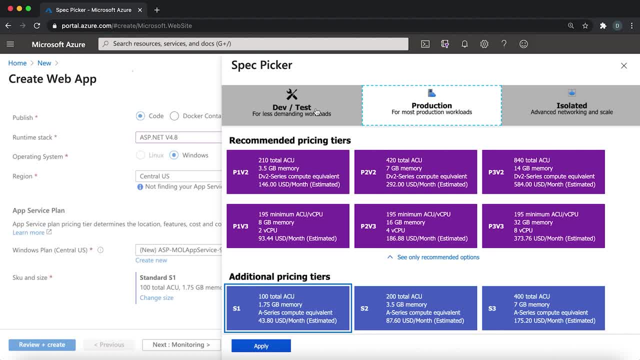 And then let's start again with this one, And the other one is a different one as well. Let me make a special one for the next slide, And for this let's change this one to the file name. We're going to go ahead and give it a name and we're going to change this. 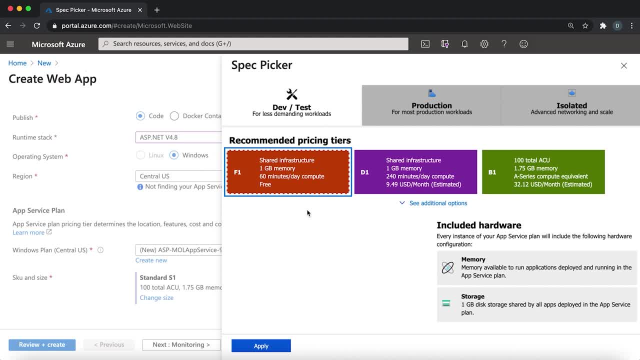 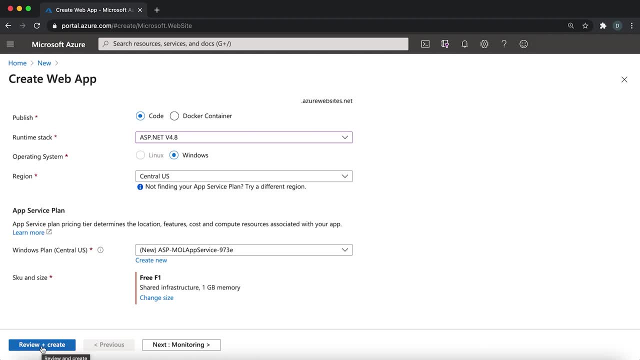 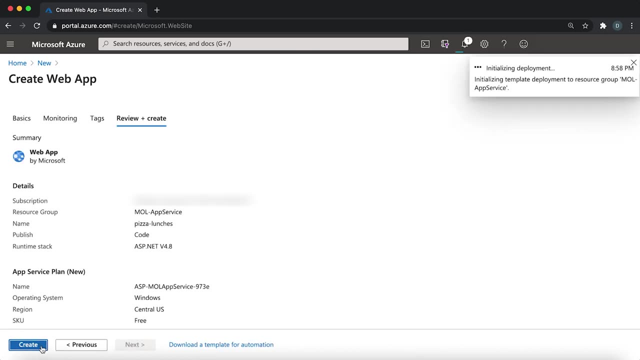 So now we have added to the process, we've created the CLM version, And let's go ahead and click save. lose any money? okay, let's click apply and click review and create, and then click create again. so now Azure is creating all the resources that you just 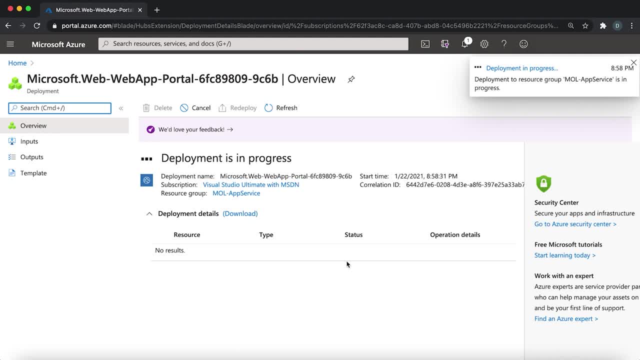 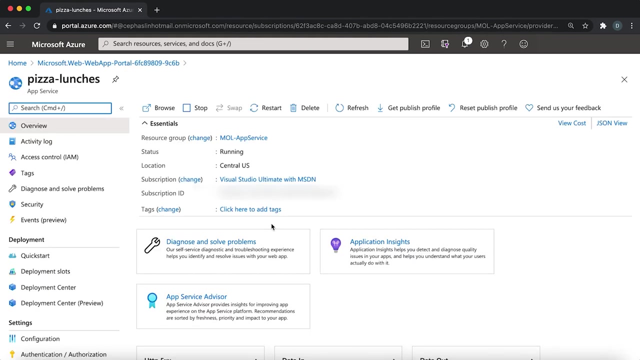 specified. that includes the resource group, the app service plan with a free pricing tier and also the app service app, and just give it a second. once you see this message that says that your deployment is complete, click on this go-to resource, which will automatically take you to the management page for your 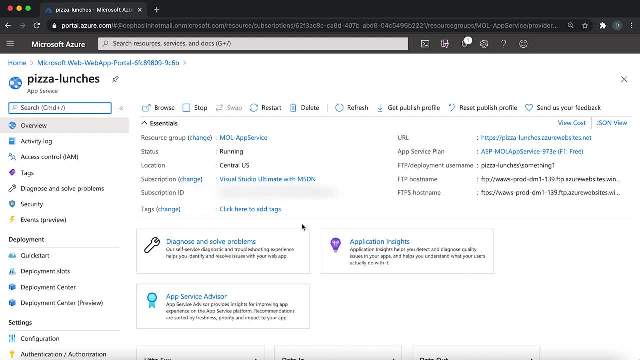 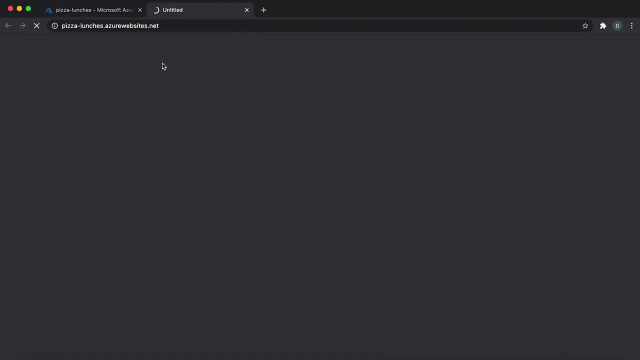 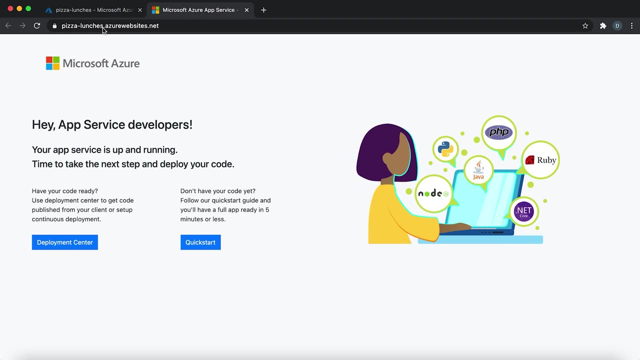 new app, service app, and then go here to the URL of your app and see what happens you right away. I just want to point out, if you remember the pizza dash lunches right here in the URL is the name that I chose for the web app name: the the name. 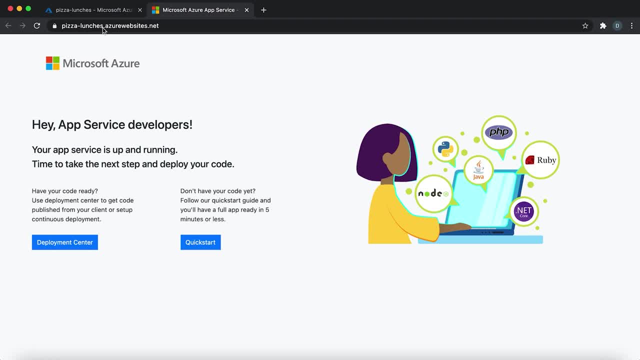 that you choose for the web app name is part of the URL, so you want to make sure that it's unique. but great, now you see a splash page that means something is running in Azure, so there. so here you can see the name. let me just tell you literally. so I made that mark up. 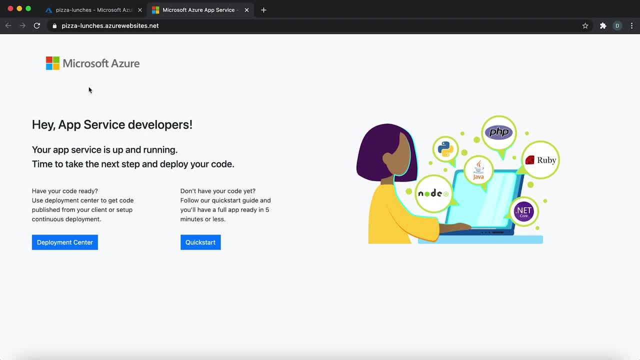 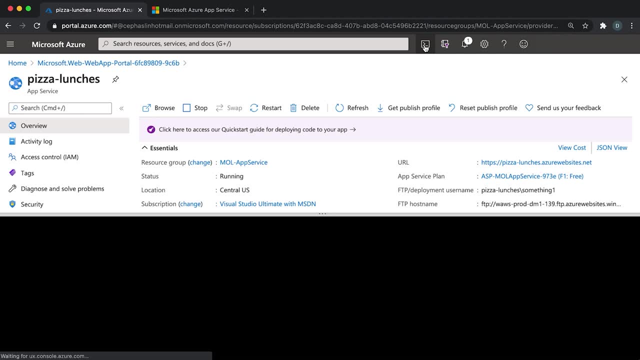 here, for here that means my code is in于 web app bank and it links into the Web Appès here. that is the file where your code roughly takes into account the two tools I showed you earlier. a lot of stuff, but this is whatños, what you're going to do next. so that's where you're going to do next. you're going to download. 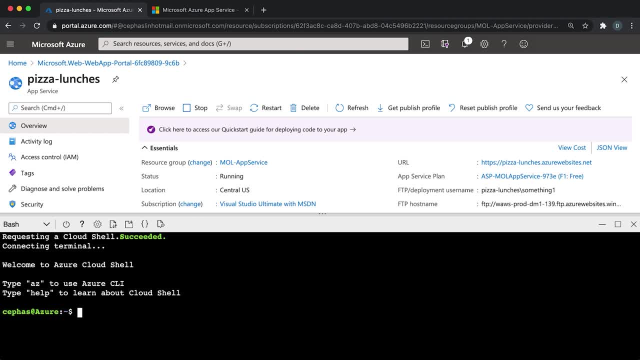 inside your browser and you can. you can run it anywhere because it's in the browser and there are two variants: one is bash and the other one is PowerShell, and for this video we're gonna stick with bash. this special is in your browser is great, because not only can you run all the Azure CLI commands, 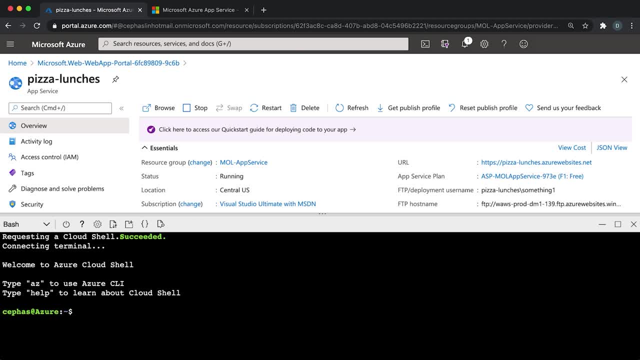 to manage your resources, but it also comes with a lot of great tools, including git, because the sample code you want is in git and it's in github. you're gonna use git to bring it down to your local folder. local means local to your cloud shell. okay, so let's paste this command called git clone and with 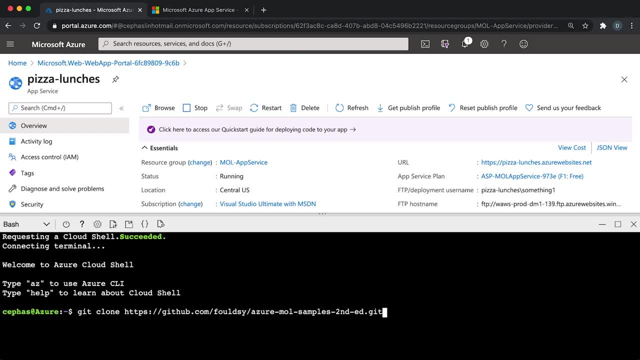 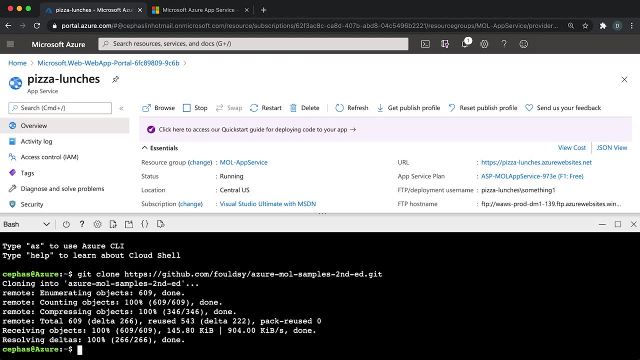 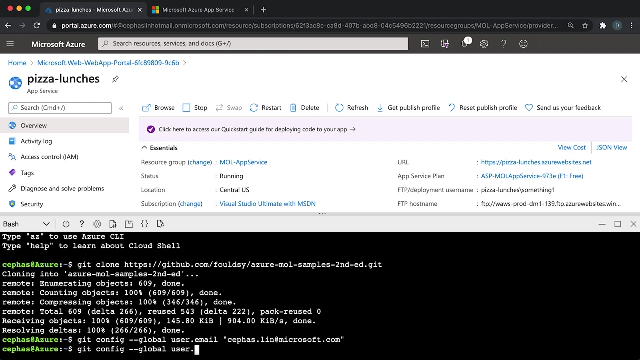 this URL to our github repo. great so, but before we move on, you, if this is your first time running git inside the cloud shell, you're gonna need to tell git who you are. so let's run git config- global user email, and then here I'm just gonna use my own, and then you have to run git config- global user name. 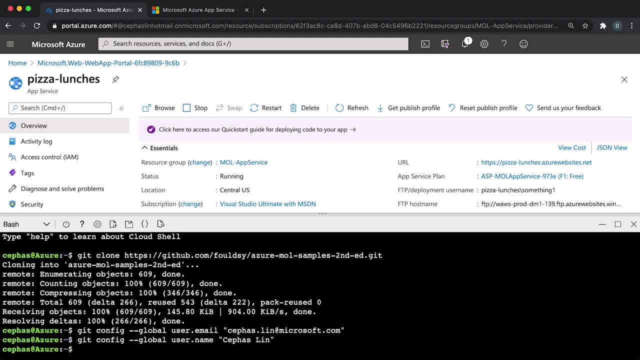 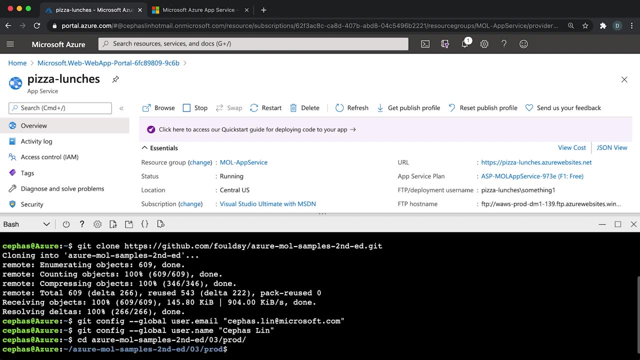 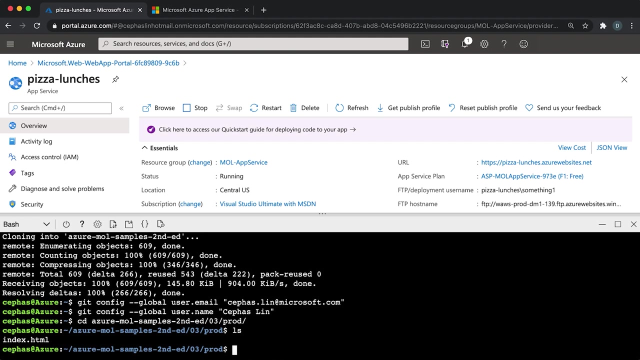 and, yes, git is a title and we're going to use the open git, Thomas. okay, so now your git installation is configured. let's go see our sample code. let's go the CD into the repository and into the third module and the prod folder. let's take a look at what's here. that's it. that's our quote quote website. that's just one HTML page, which is kind of perfect. bit of an exception. so I did an html code review on it to see if there might be any important things. but for the content into the app we don't want to let this crt tool it just be a copes with the file paste here. if you didn't notice that here, there's a body of pins there which are almost everywhere that are alltense multiplier. 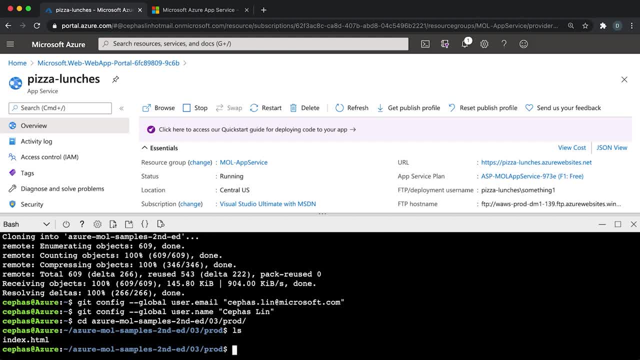 page which is kind of simplistic, but you can kind of imagine if you have a Nodejs app in this folder or a Python app in this folder, you would use the same steps to deploy them. So you have a folder with some files, or here a file, but in order to deploy it to your 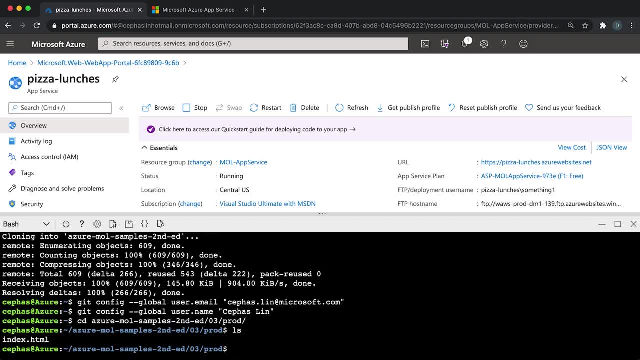 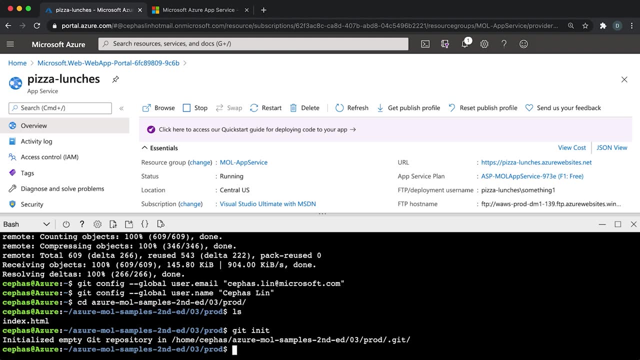 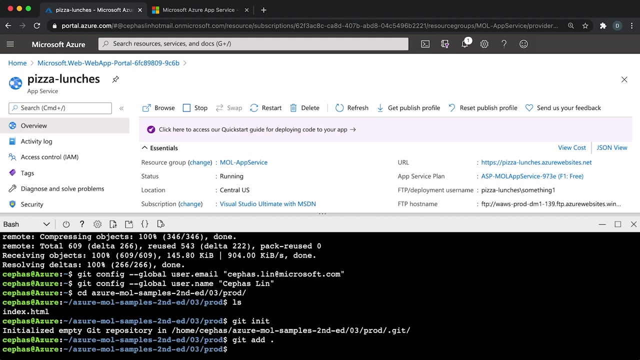 app service app with Git. this needs to be a Git repository. So let's initialize a Git repository using git init And then, once we have this initialized Git repository, let's add the files to it. Git add period: The add period adds all the files in this folder into the repository. 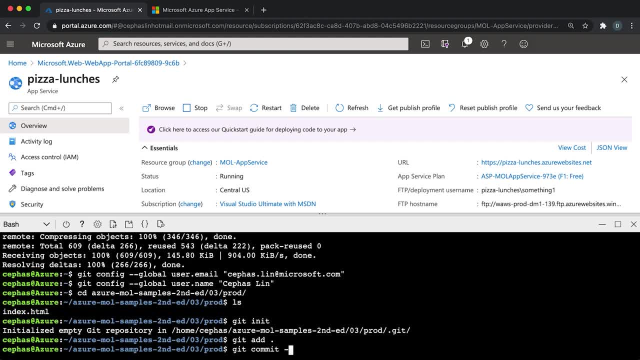 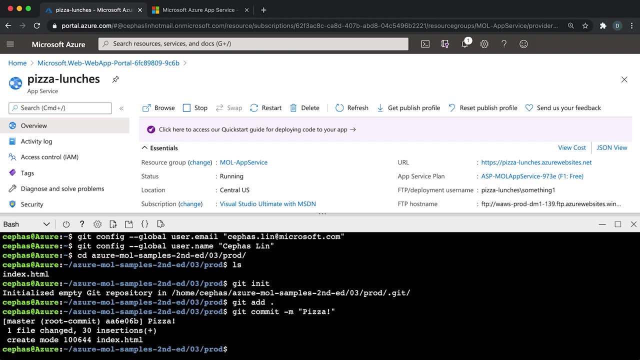 Now, once we add them, we need to commit our changes. Let's have a Nice commit message: pizza. So this Git repository is ready to go. However, on the app service side, for pizza lunches app service app, this app by default. 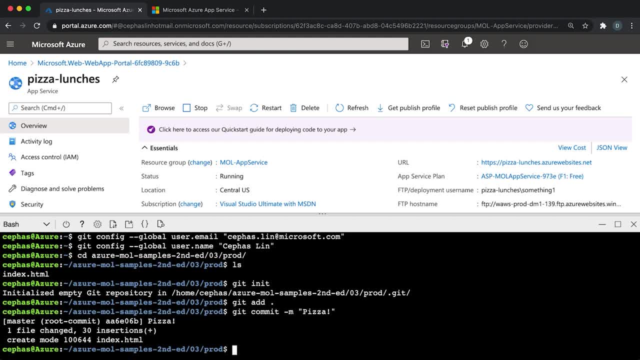 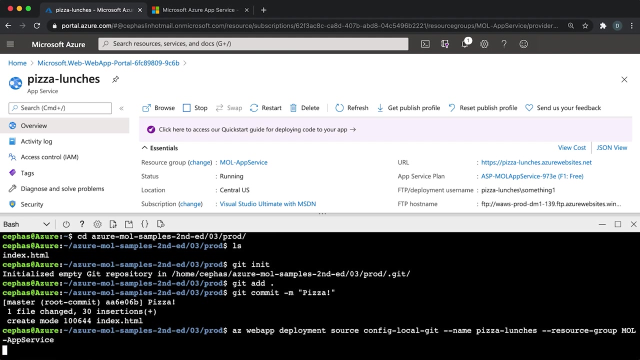 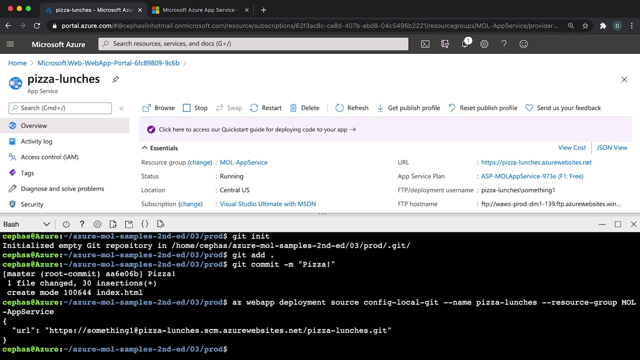 does not accept Git deployment yet, And so you need to configure that. So you're going to run az webapp deployment source config And then give it a name of your app, which is pizza lunches, And also the resource group name. So this command outputs a URL that you can use for your Git deployment, but what's embedded? 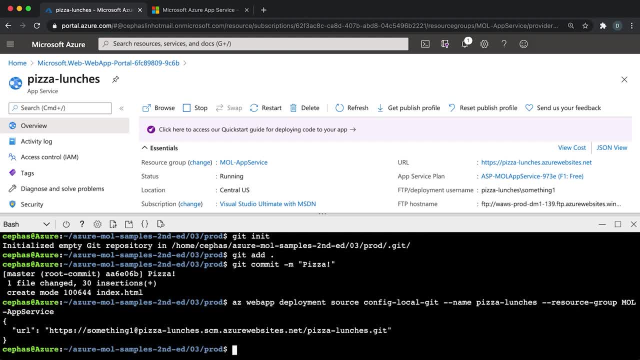 in it Is the user level credentials And if you read the book, the book tells you to use the user level credentials to deploy your app. But in this video I want to show you how to use the app level credentials. The user level and app level credentials are both both credentials that you can use to 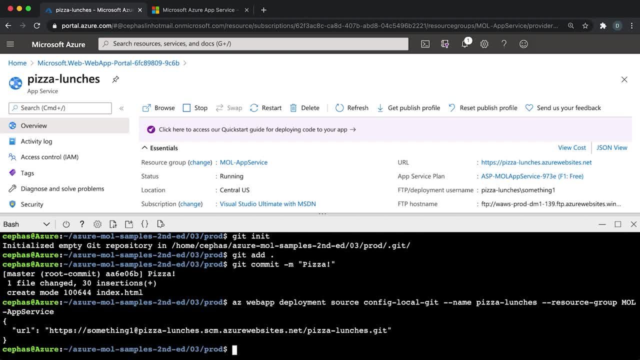 deploy your code to an app service app. The difference is that the user level credentials can be used to deploy code to any app in your subscription, Whereas the app level credentials can only be used for that particular app, And so, in a sense, you can say that the user level credentials are more convenient, while 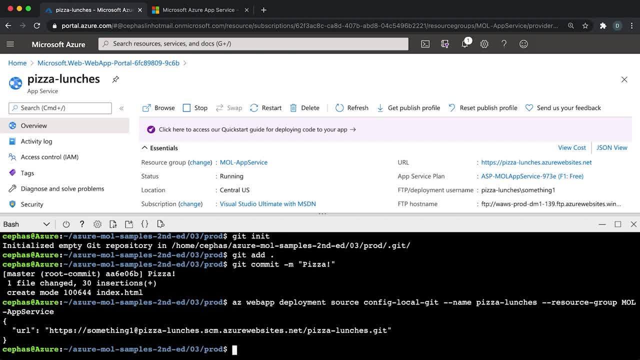 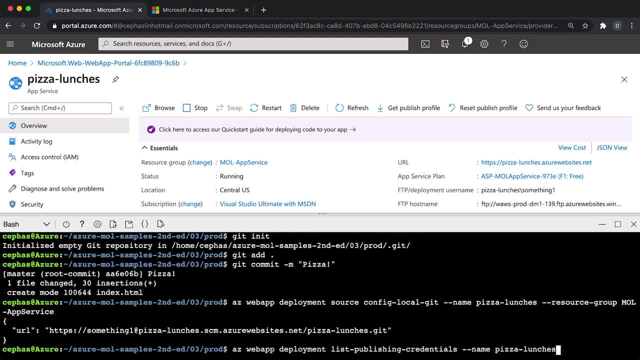 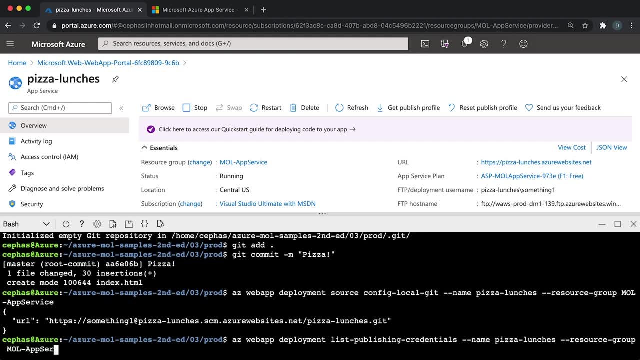 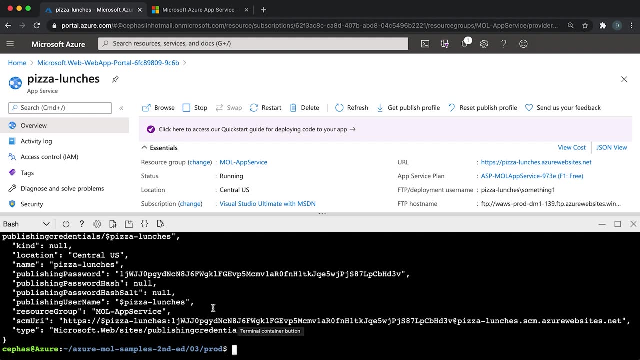 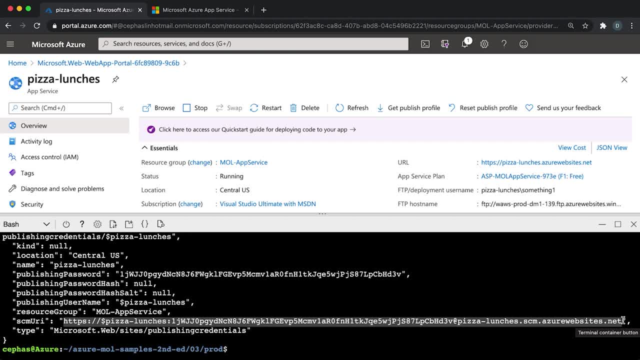 for you for your deployment. that has the username and the password already embedded. We're going to copy this And then we're going to add this as a remote into your local GitHub repository. So let's do git remote, add Azure. That means add a remote to this Git repository called Azure. 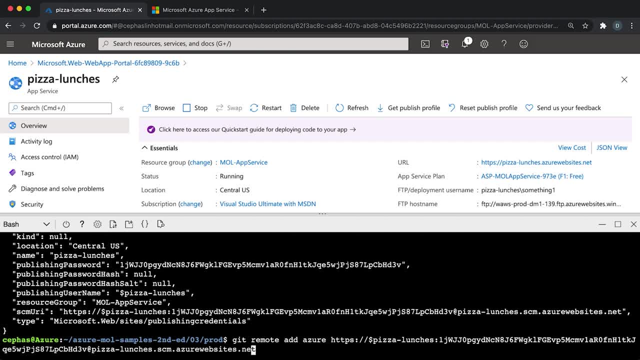 And we're going to paste this URL. Don't run this yet, because, notice here, this $pizza is going to be interpreted by Bash as a variable, And we don't want to. we don't want Bash to do that, So we're going to work around it by adding a single quotes. 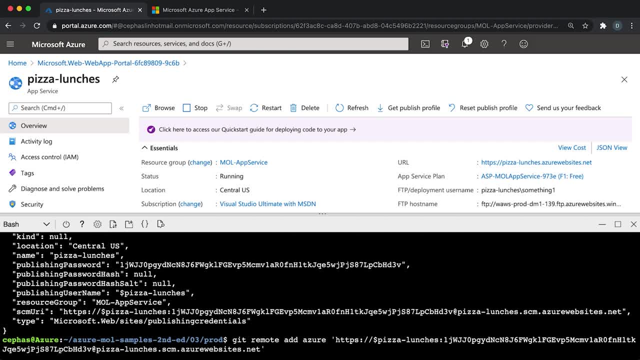 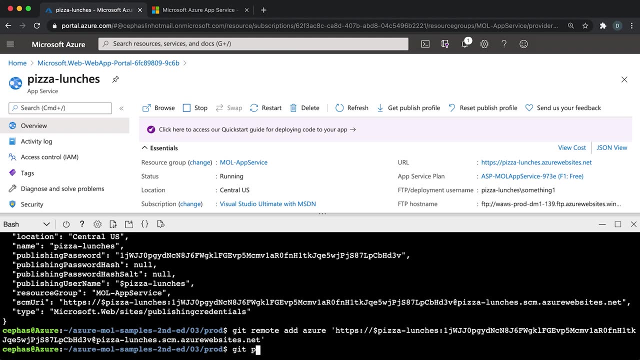 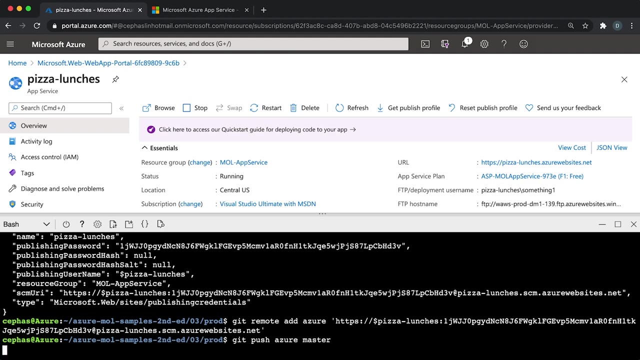 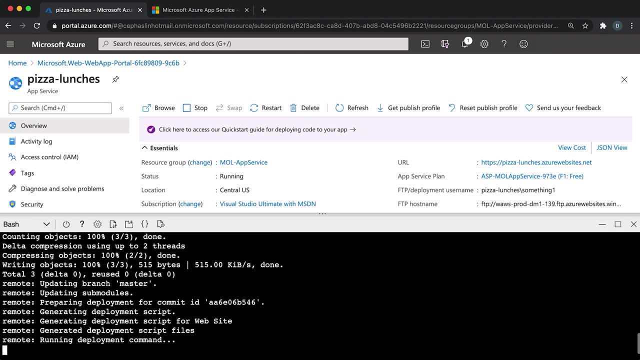 And the single quotes will make sure that Bash interprets that character just as a dollar sign character. OK, So now you just need to do a git push to that remote Push Azure master. Great, That's it. The code is deployed. 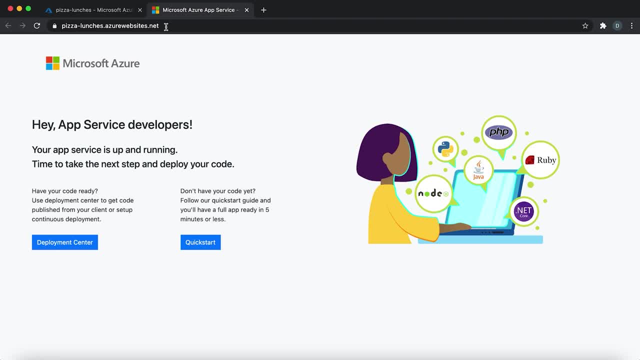 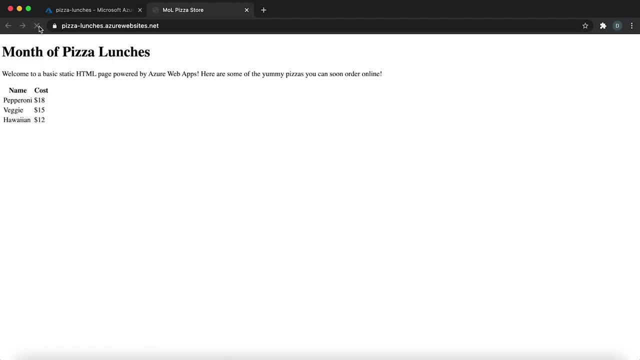 So you just go back to the web page and refresh it. Wonderful. Now you see that the HTML file is deployed and it's displayed at the URL. This is great, but what if I tell you that you can do all the things that we just 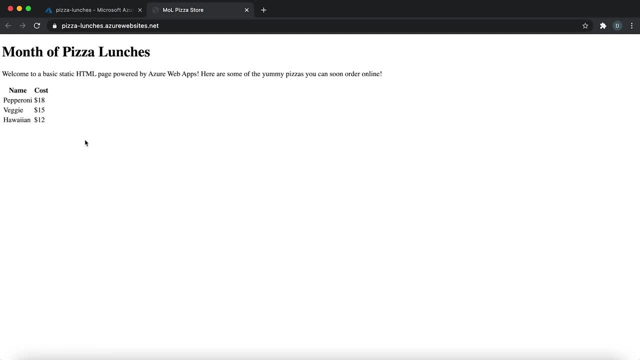 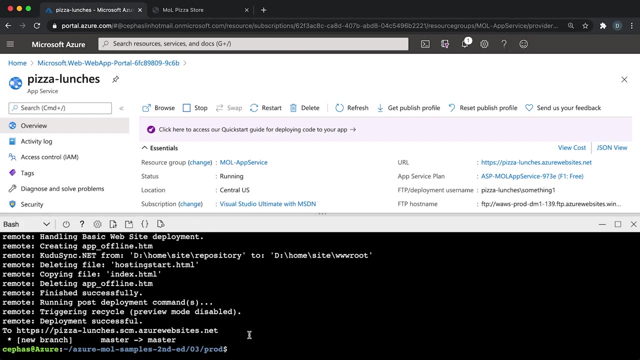 did, including creating the resources and pushing your code to Azure with just one single Azure CLI command, And I want to show you right now. So if you go back to the Azure portal, back to the Azure Cloud Shell, let's assume that you're already in the folder. 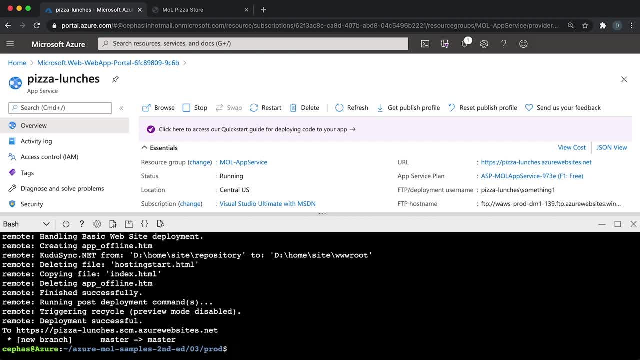 that you want to deploy, and then you haven't deployed any resources yet. So let's run azweb webapp up And let's give it a different name, called pizza lunches quick, because it's quicker, And then let's add a HTML flag. 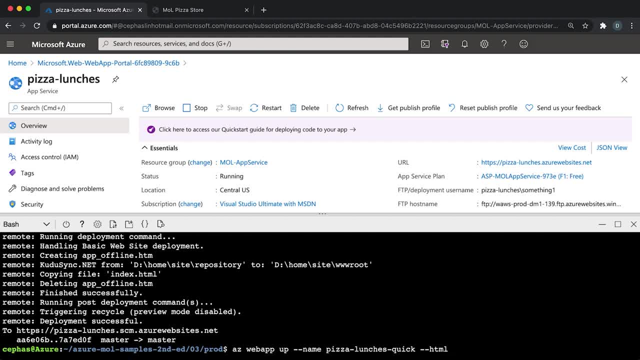 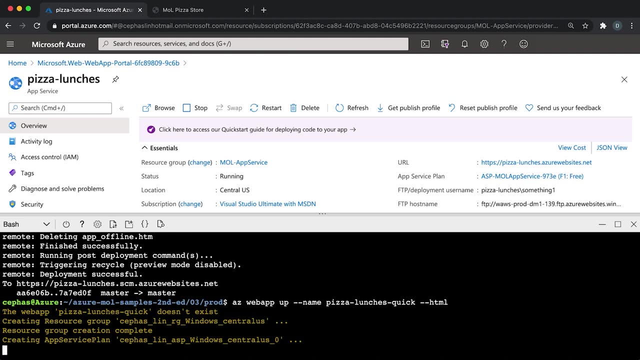 This tells the hdwebapp up command not to try to interpret the files that are in the folder, because those are just HTML files. OK, So let's run it So immediately. the azwebapp up command recognizes that the web app called pizza lunches quick. 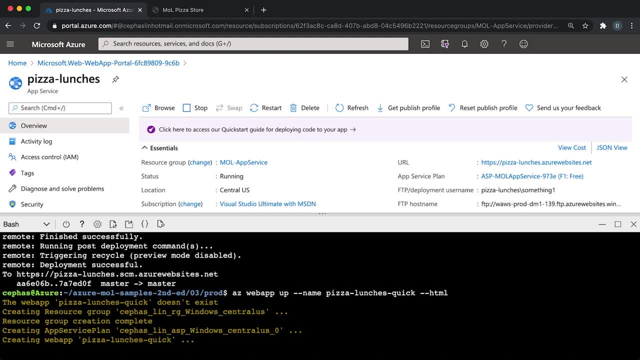 doesn't exist. So it tries to create a resource group for it and an app service plan for it and the app service app for it And once the resources are created, it will try to zip up all the content of the folder and then upload it as a zip package, which is what 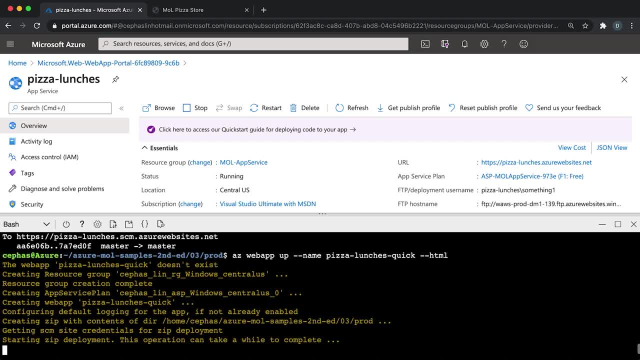 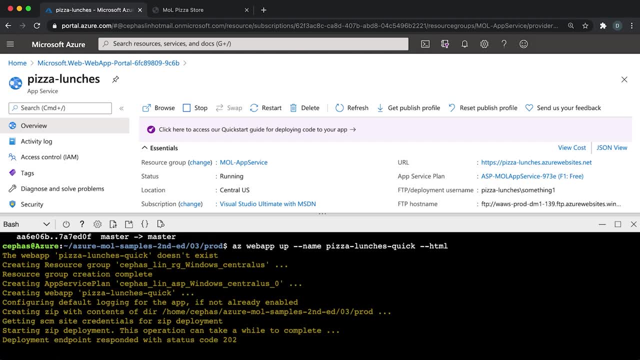 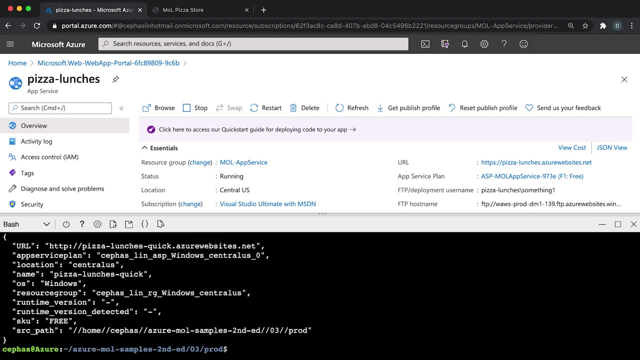 it's about to do right now, See, And so the nice thing about this approach is that you don't even need Git and you don't even need to play around with publishing credentials, because that one command does all of that for you. OK. 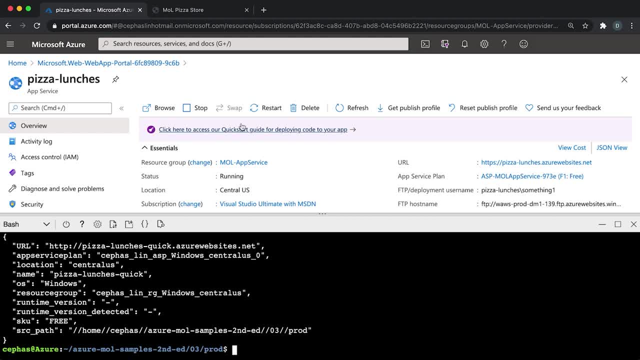 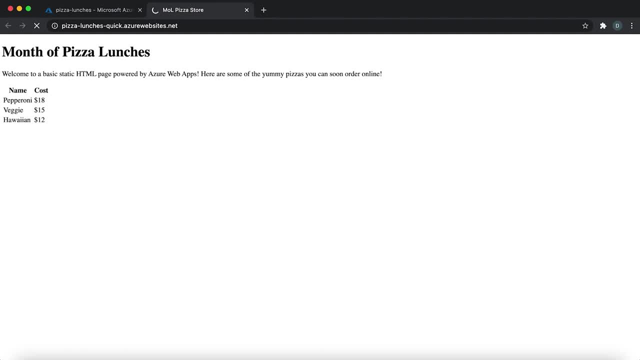 So now the app is deployed, Let's go to pizza lunches quick And let's see what happens. Great, Same result. The HTML file is deployed to this new app and it doesn't take that many steps, just one step. You can imagine that, of course, this. 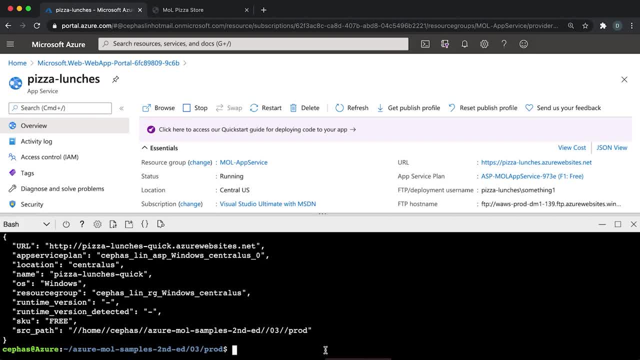 is done in Azure Cloud Shell. But if you were on your own development machine and you have an app in this one folder that you want to deploy, you just need to install Azure CLI on your local machine. OK, And then you can just use azwebapp up to deploy. 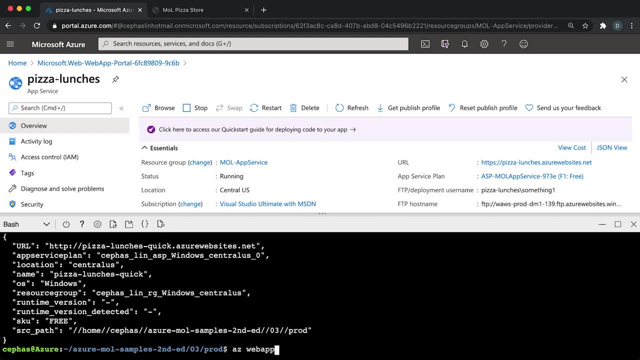 And let's say you make any changes and then you want to redeploy your app, you just run the same command And you don't even need to specify the resource group or the app service plan or the app name again, because the first time you ran the command. 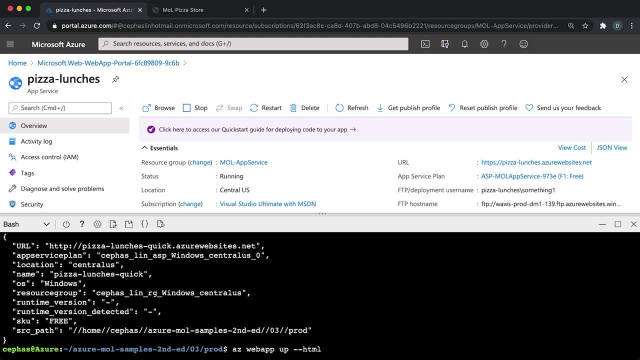 azwebapp up already, remembered it and then stored it into your local folder, And so now, any time that you want to redeploy, you just run azwebapp up. OK, Just run azwebapp up like that, And, of course, if you have something other than HTML, 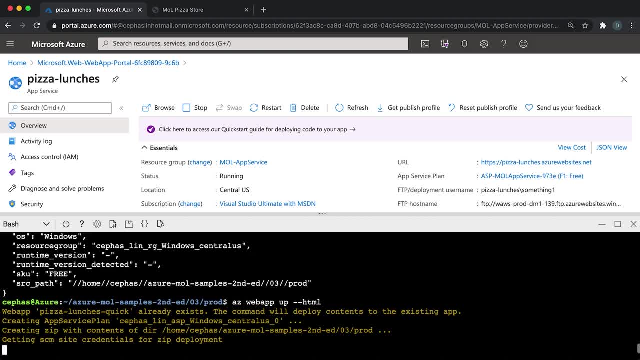 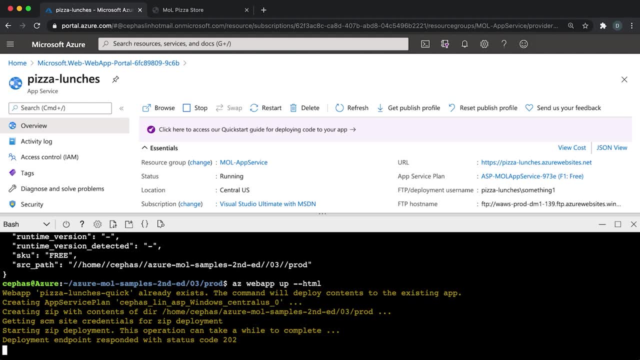 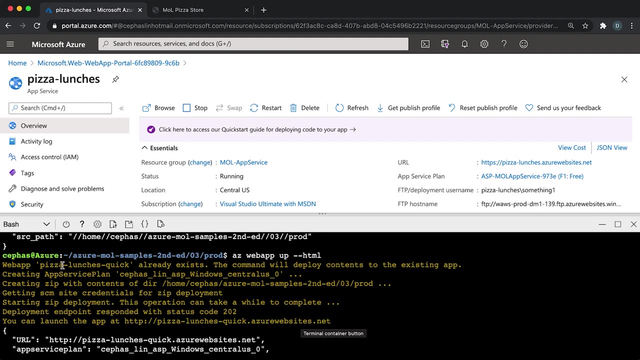 then you would just run that. You would just run it without the HTML flag And of course I don't expect anything to change here. I'm just showing you that that's all you need to do to redeploy And the command recognizes that the Pizza Lunches Quick app. 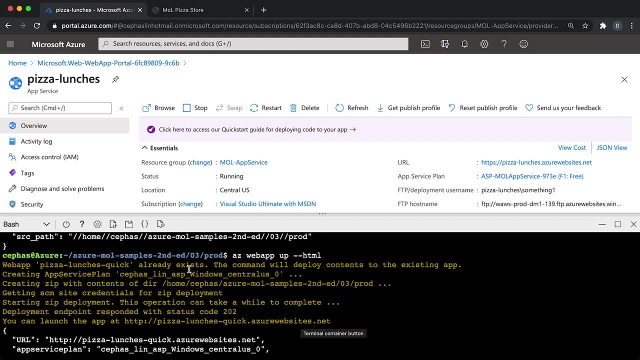 already exists, And so it's not going to try to create any resources, And it will just try to Perform another zip deployment. So great. This is the end of the demo. I showed you two different ways to deploy a simple HTML site to Azure App Service. 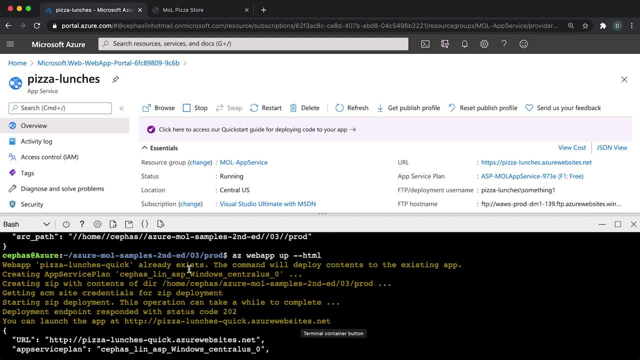 You may ask: which way should I choose? That's really a preference matter. You may be already using GitHub to do source code management, in which case a Git deployment would really make sense, But if not, then azwebapp up may offer you a very easy way. 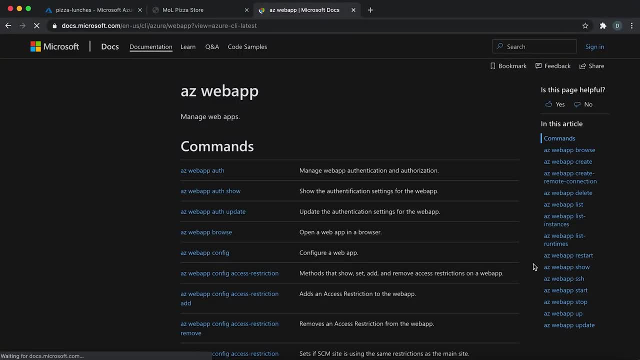 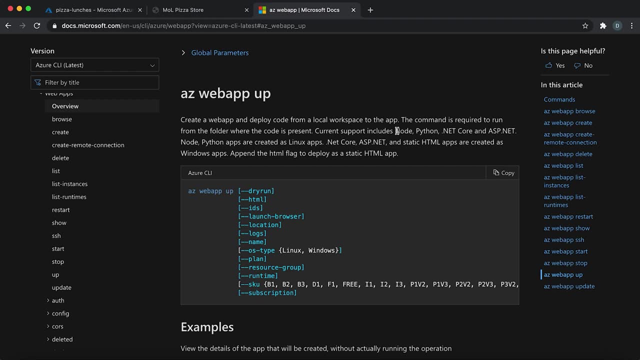 azwebapp up. it doesn't support all the language runtimes Right now. according to the documentation, it only supports Node Python, NET Core and ASPNET, So it may factor into your decision whether to choose azwebapp up. 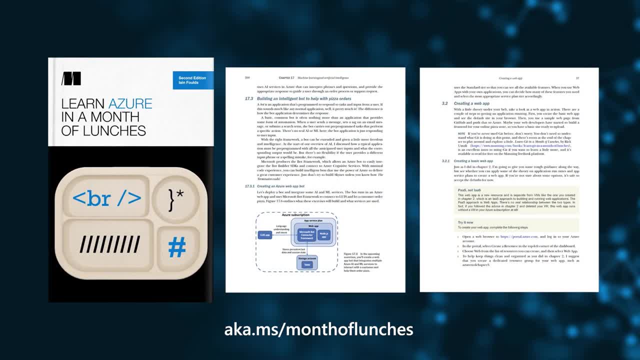 If you enjoyed this tutorial, the e-book has even more examples waiting for you to work through. Download your free copy of Learn Azure in a month of lunches.